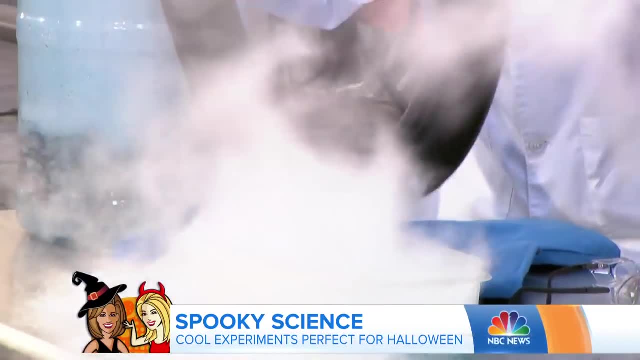 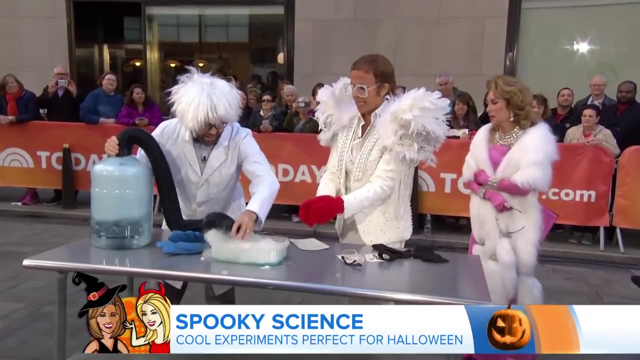 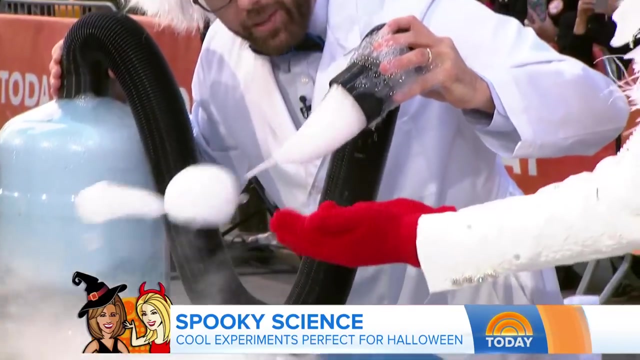 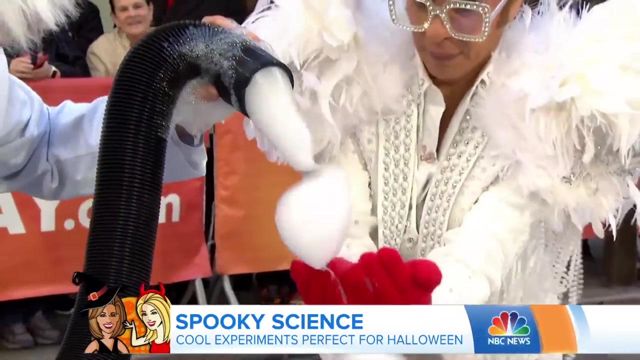 all Halloween is is a bunch of science. What am I doing? We'll see. It's a little windy here on the plaza. We'll see if we can make this work. But you'll notice how the wind as it blows. Yeah, I see It's like a big blob. It's a big blob. Oh, I see. I see, Let me mix it up one more time, Okay, And then we'll hold it like that and look at that. Pretty cool. You'll notice as the wind carries it away. That's cool. Ghosts in a bubble, That is cool. Here we go again, And if you catch it just right, without the wind interrupting our science experiment, I thought that was cool. That is really cool. 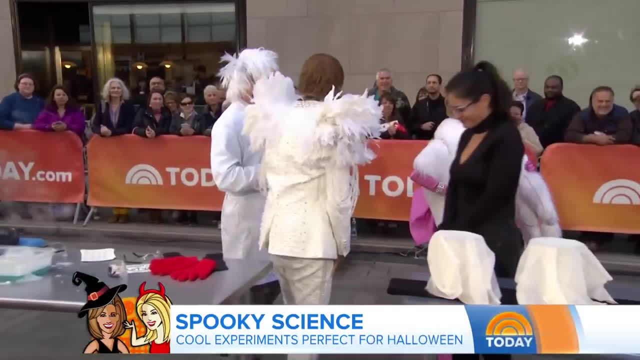 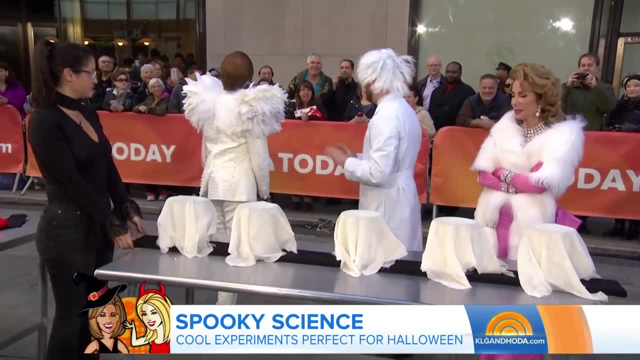 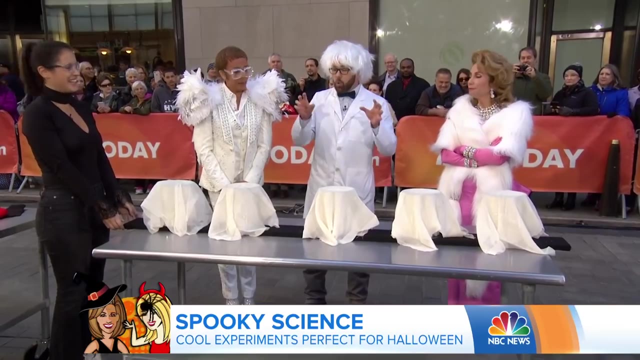 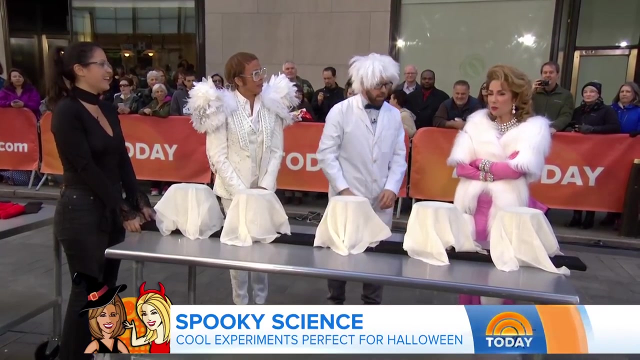 Amazing. right Now, over here, we're going to make these ghosts fly through the air. I want everybody to know that the loud noise you hear like a balloon is that popping. It is nothing else other than just a little bang going up into the air like a balloon Inside two ingredients. We're going to mix those ingredients together. A chemical reaction will happen And this should send our ghosts flying through the air. Good, That's where they should go. Close your eyes, Kathy. Donna over here is going to hold that side. I can't get them through the wig glue. I'm going to hold this. 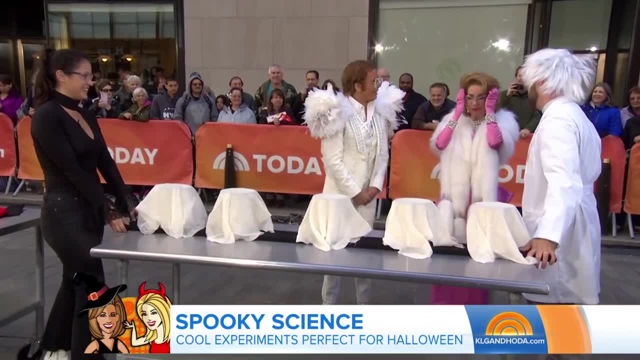 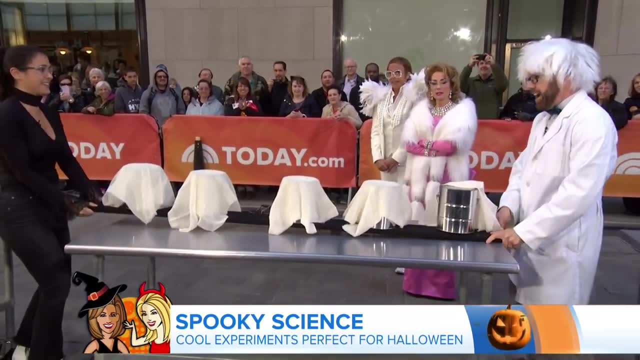 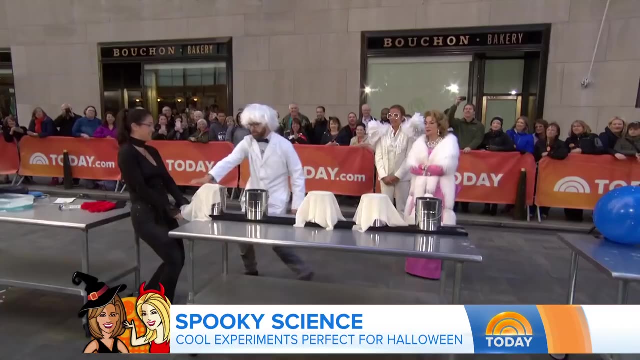 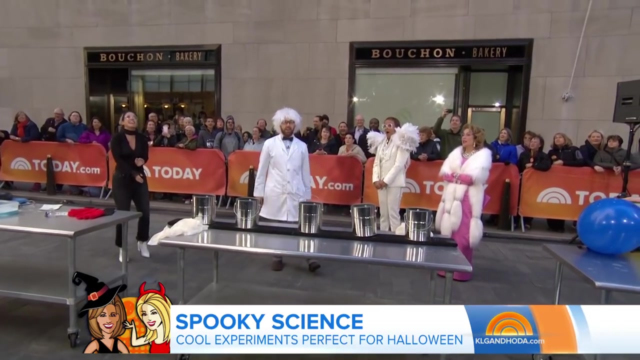 Put them on the outside. Just put them on the outside. Okay, On the outside. Yeah, like that, Scoot back for me for your safety. Are you ready, Donna? What's happening? Okay, And just keep shaking. There we go, There we go, You got it. Step back, Donna, You're good, Step back, Step back, You're good, Step back. So what's happening is we have our ghosts flying through the air. Cool, Awesome, That was cool. Awesome, That was cool. 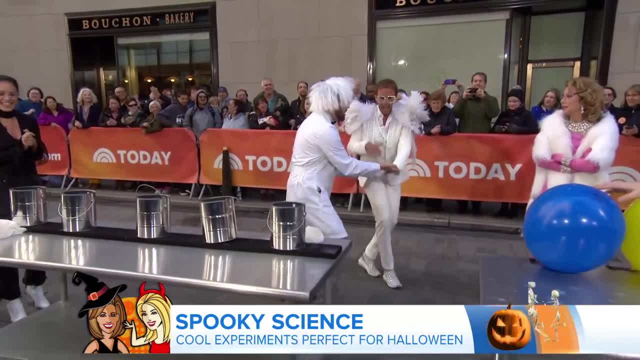 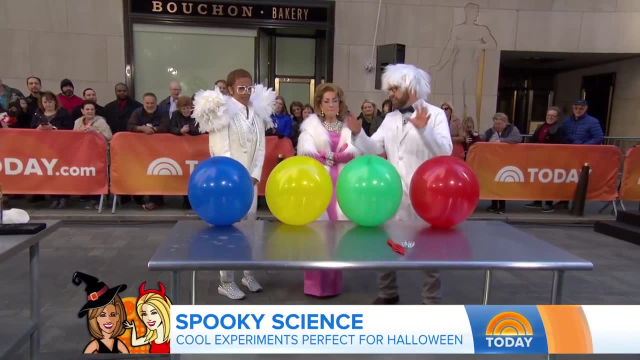 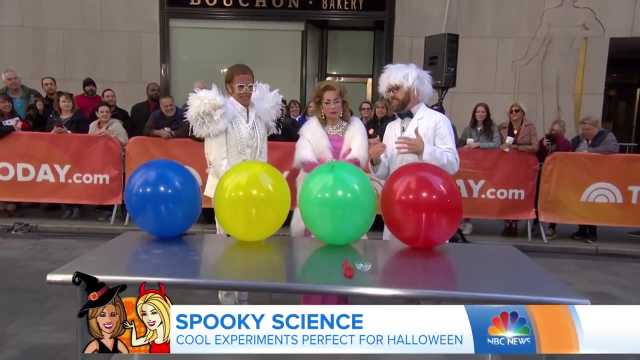 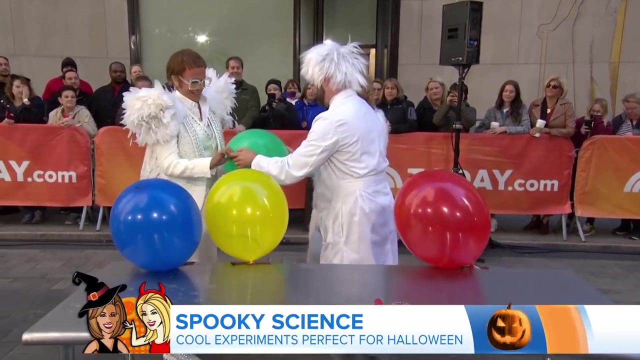 Science. That was awesome. Five for science, ladies, Quickly, Yes, Yes, Yes, Yes, Okay. How are you guys Good? Okay, Okay, These here. we have a ghost inside. This is an experiment you can do at home. Okay, There is a hex nut on the inside. A hex nut has six sides. It's going to rub against the sides of the balloon and it's going to create a unique sound. So I'm going to undo the green one. You hold this one, just like that, on each side, just like I'm holding it. Which color would you like? Kathy? I'll take the yellow. The yellow, just for you.